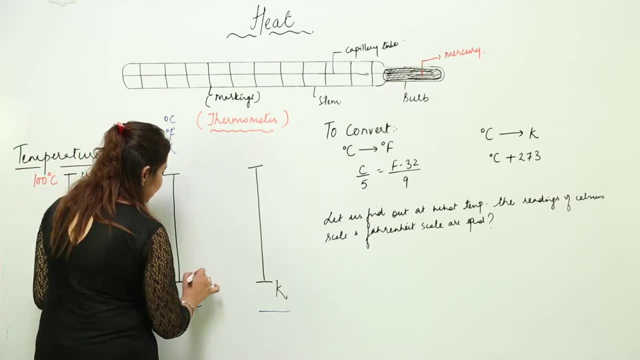 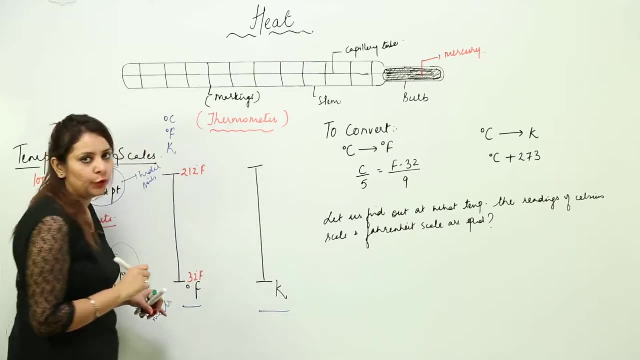 Same for in Farad. like in Farad, what we have it is 32 degree Farad is the lower fixed point and 212 degree Farad is the upper fixed point. That is at which the ice melts, And this is at what the water boils. 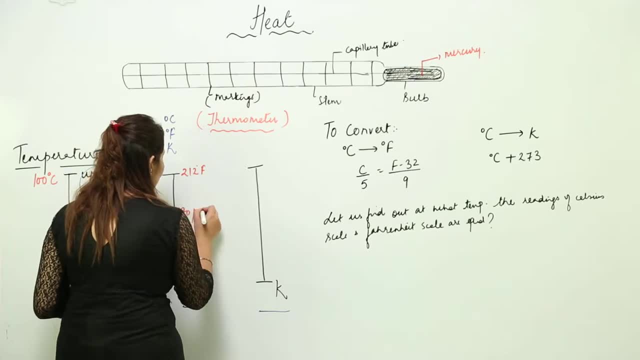 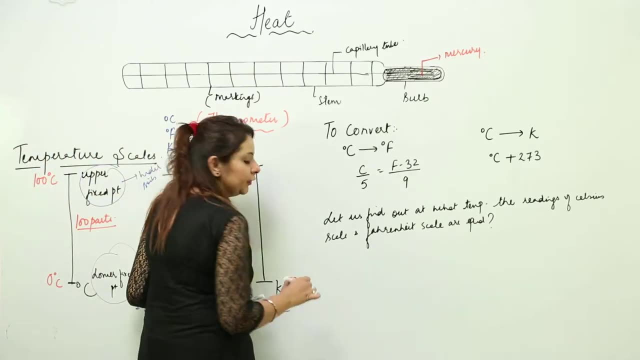 And it is actually divided into equally, into 180 parts And if we look for the Kelvin, the lower fixed point is 273, lower fixed point or lower fixed temperature at which the ice melts, And the upper fixed point is 373 Kelvin. 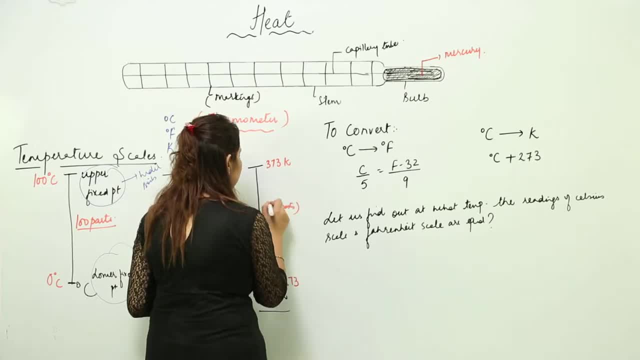 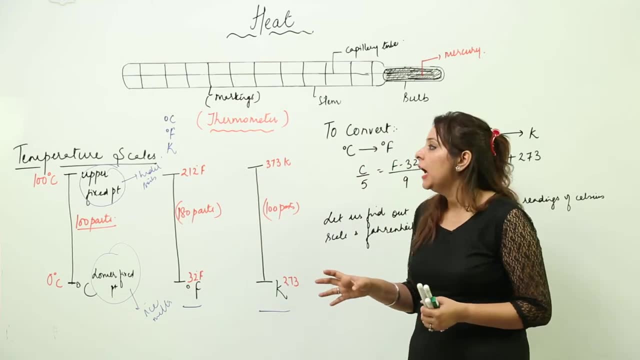 So again it is divided into 100 parts. So these are the temperature scales. You need to remember the lower fixed point and the upper fixed point on all of these scales And you know that we can actually convert the temperature on one temperature scale to another. 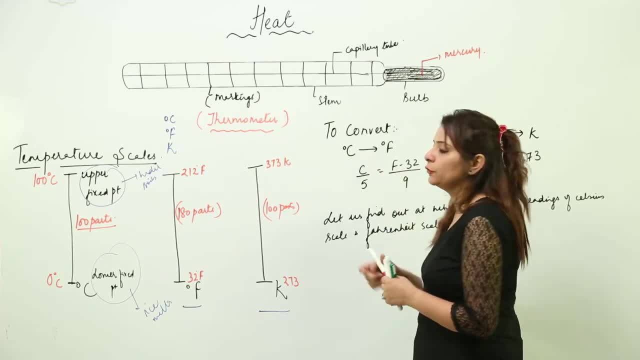 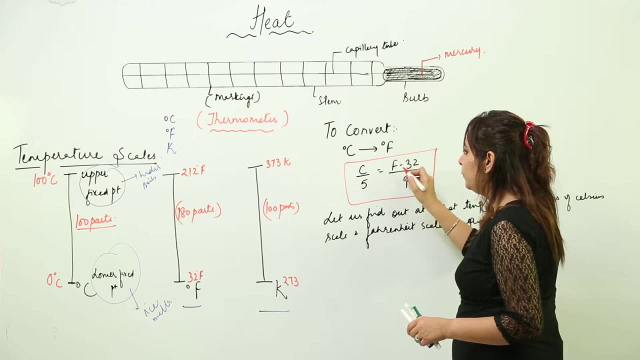 Suppose, if you wish to convert degree Celsius into Farad, then what formula you will be using? You will be using this one: C upon 5 is equal to F minus 32 upon 9.. Suppose, if you have temperature 100 degree Celsius and you need to convert into Farad, 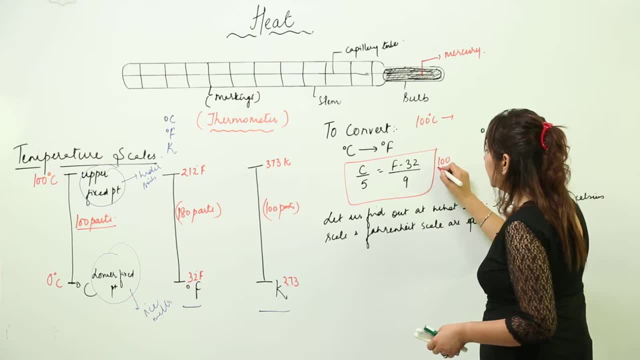 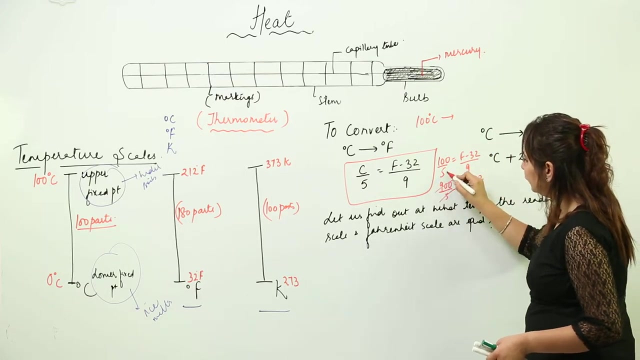 So how you will be doing that? You will be doing that 100 upon 5 is equal to F minus 32 upon 9.. Comes out to be: 900 upon 5 is equal to F minus 32.. Or if you solve for it 5, 1 to 5, it comes out to be 180. 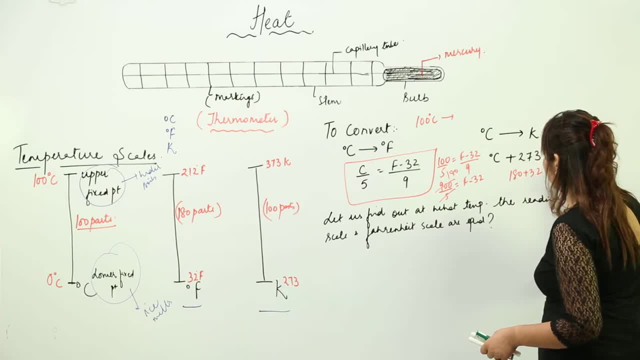 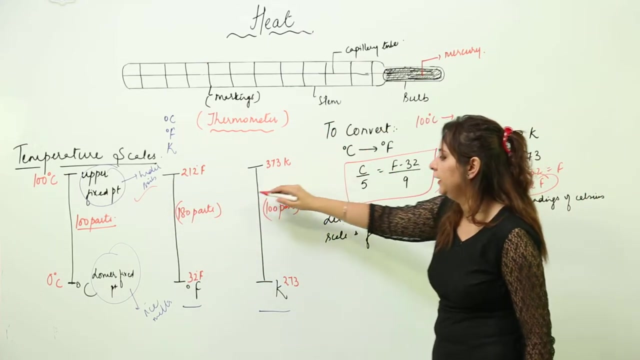 So it is 180 plus 32 is equal to Farad. Because this comes here, it becomes plus, So it comes out to be 2212 Farad. Again. you know that 100 is the upper fixed point And upper fixed point on the Farad is 212. 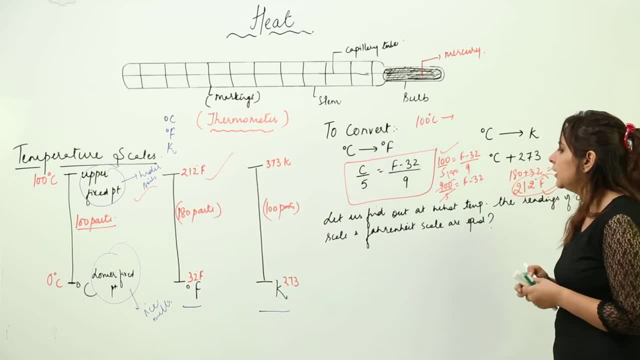 So same answer: 212 degree Farad. So if you get a question like this, let us find out that at what temperature the reading on the degree Celsius and Farad is going to be same. So how you will be doing that: You will consider temperature as x. 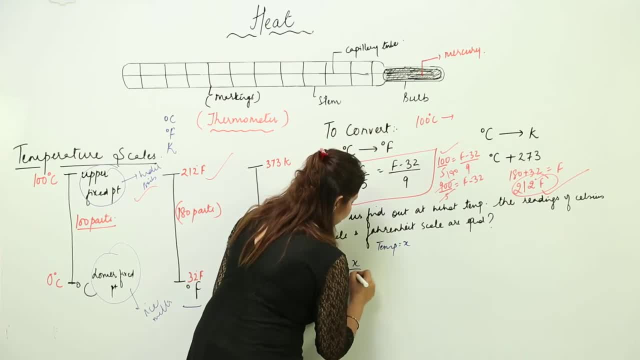 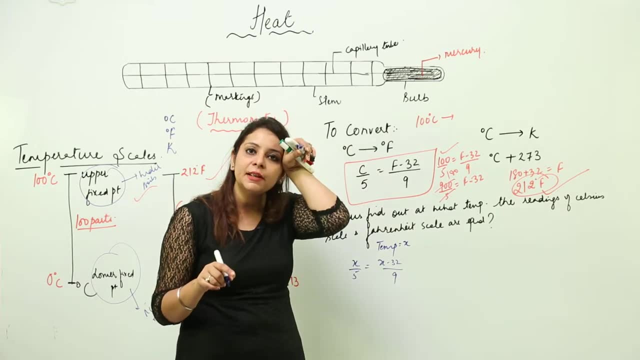 Putting in it, you have x upon 5, x minus 32 upon 9.. Because we are taking temperature on Celsius and Farad, both at x, Suppose we say that at temperature x they both are equal. So I have taken x.